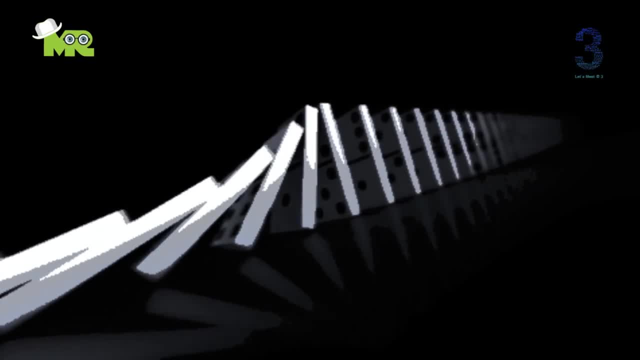 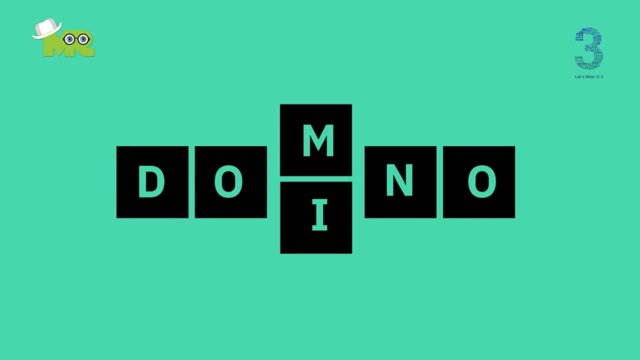 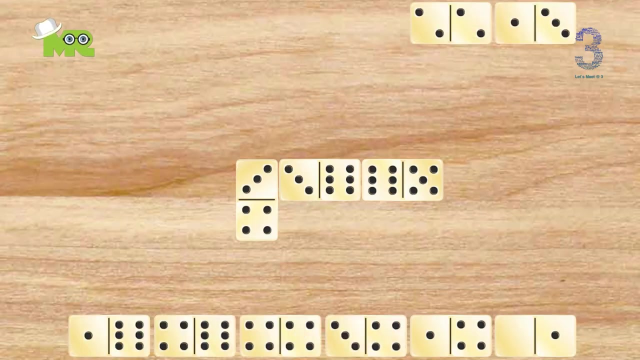 Domino's is a relatively simple game. however, there are a few general strategies to keep in mind when playing. If you are playing the block and draw a Domino's game, here are some useful tips. Try to keep a variety of tiles. Try to keep as many different tiles in your hand as long as possible. This will help you. 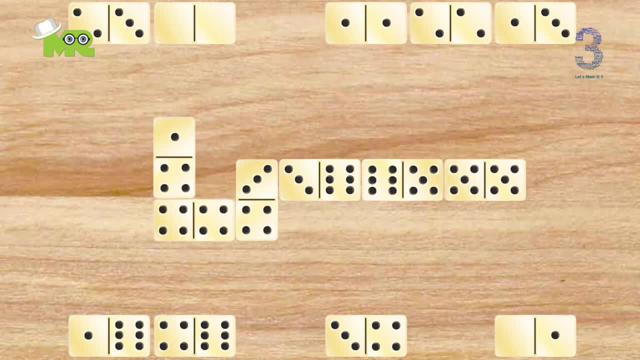 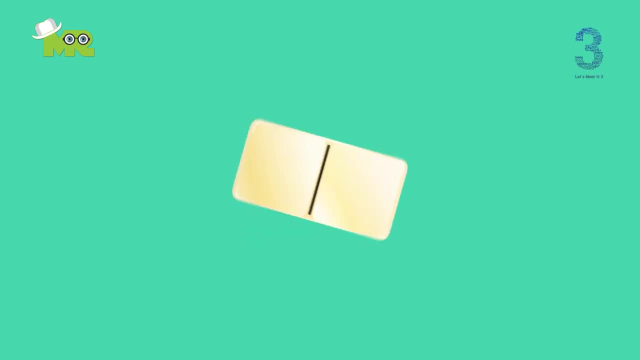 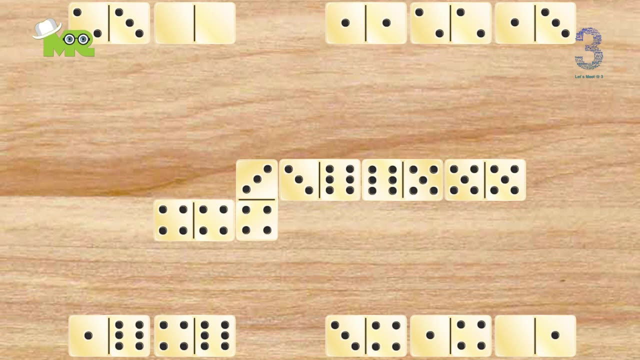 keep from getting stuck in an unplayable position. Always try to play doubles early, Because doubles have the same tile value on both sides. you will have fewer opportunities to set them down in the layout, so it's a good idea to play doubles whenever you have the opportunity. 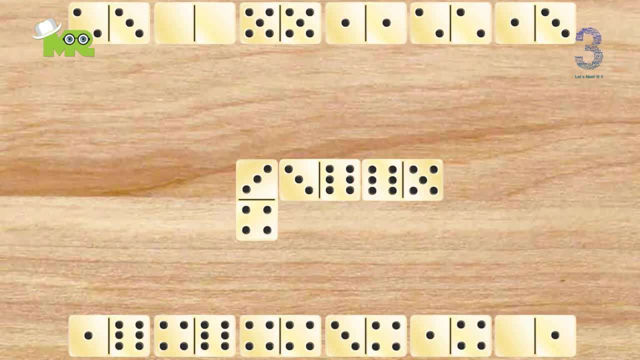 Play your heavier tiles early. You don't know for sure who will win a round of Domino's. It's a good idea to play your high-value domino tiles as soon as possible. That way, even if your opponent wins a round, hopefully they won't score too many points. 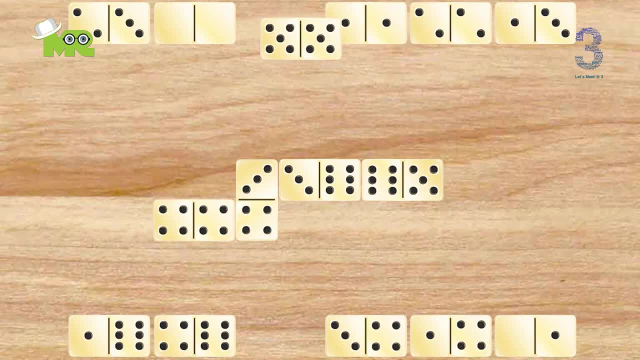 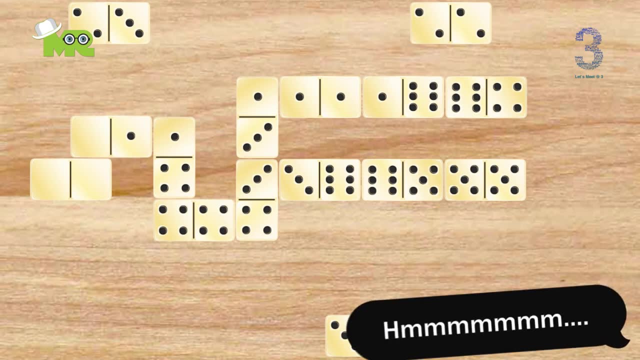 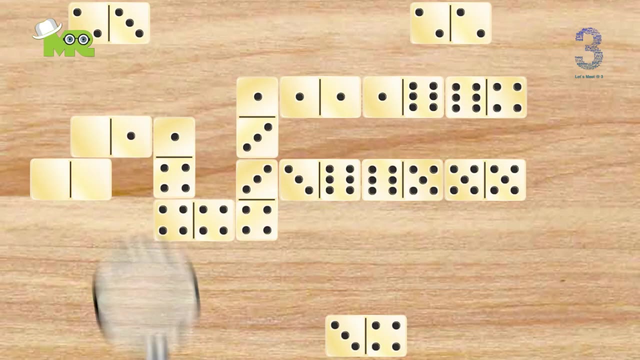 Always note your opponent's weaknesses. When your opponent has to pass or draw a tile from the Boneyard, remember which tile values they don't have. This information will help you to block them later in gameplay. Determine your opponent's tiles. If you study the 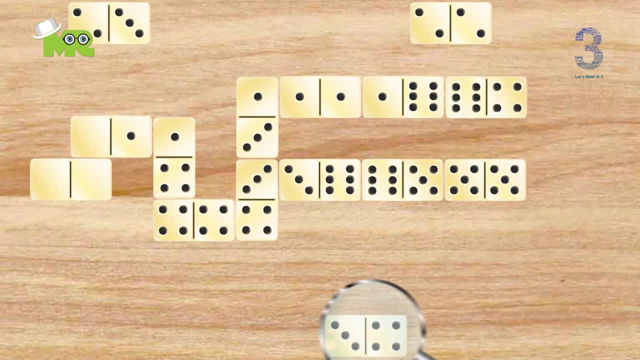 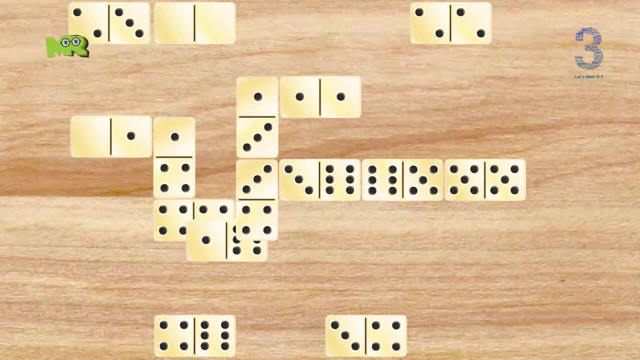 layout of already-played tiles and the tiles in your hand, you will often be able to guess what your opponents are holding in their hands. This is especially true late in the round, when most of the dominoes have been played. This information will help you to block your opponent. 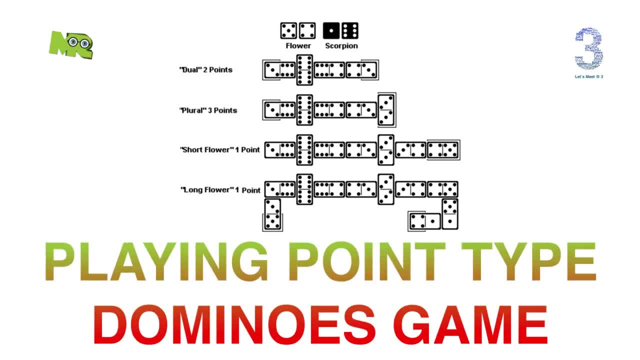 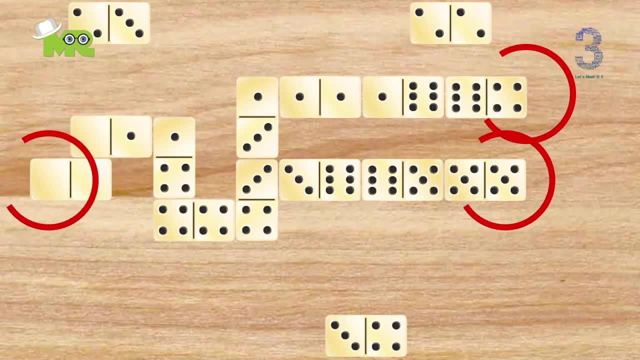 Now let's talk about if you're playing point-type dominoes game and what are useful tips. Always be aware of the board count. This is the total of all open ends on the layout. In-game, like fives, players score points when the board count is a multiple of five. Evaluate the tiles. 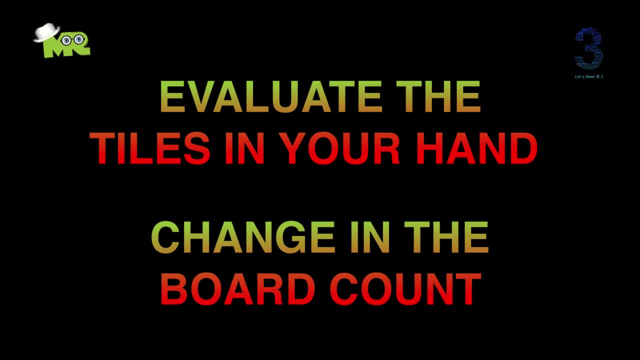 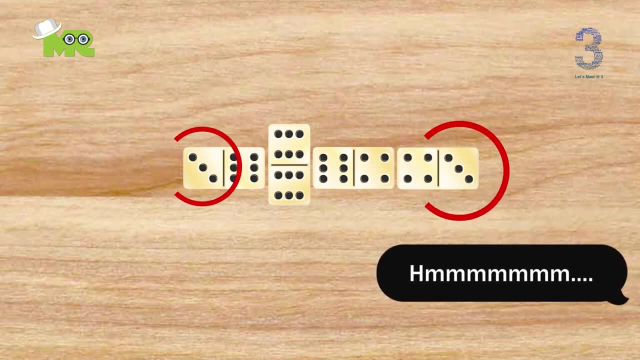 in your hand and how they can change the board count. Determine the difference between tile values on either end of the tile so you can quickly know how they will change the board count. For example, five and three on each end will change the board count by two, Connecting the. 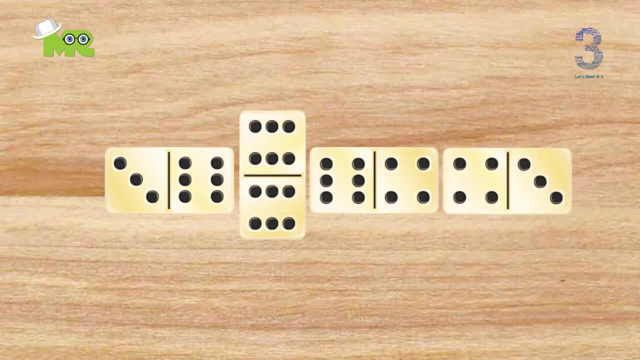 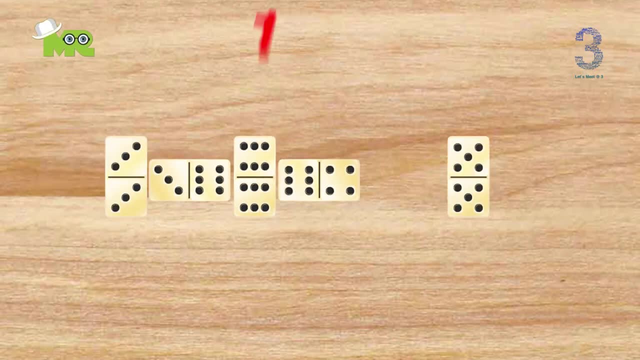 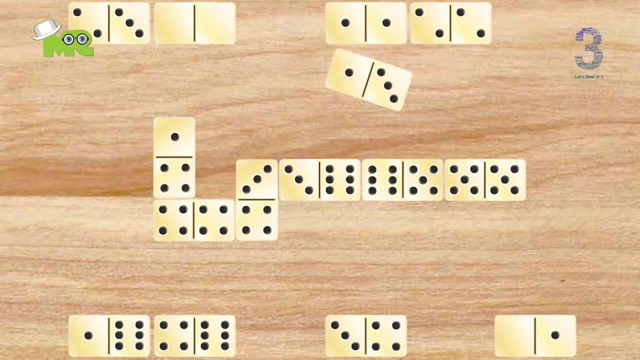 lower end to the open end of the layout will raise the board count. Use blocking strategies towards the end of the point game when the opportunity for scoring points diminish. Control and manipulate the board count In a game of fives where you score points for board counts that are multiples.